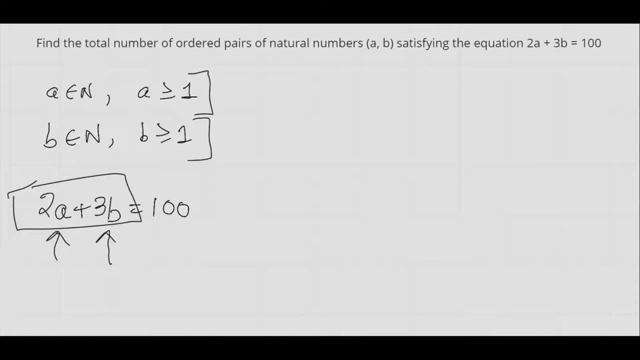 Let's find the maximum value of B, So in that case A would be 1.. So 2 into 1 plus 3b is less than equals to 100, right? So 2 plus 3b is less than equals to 100.. 3b is: 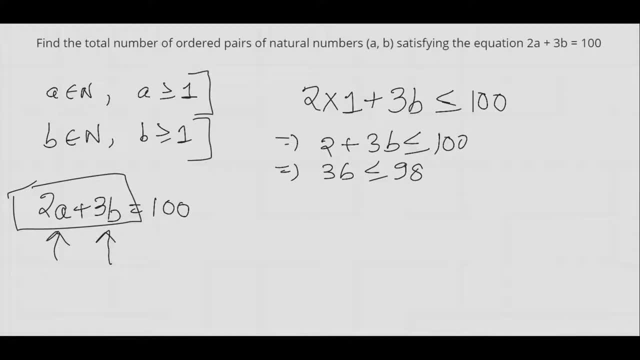 less than equals to 98.. 8. 9. take integer values, that to only positive integers. So B less than equals to 98 by 3 will round it off to the nearest integer, which in this case is 32.. So B less than. 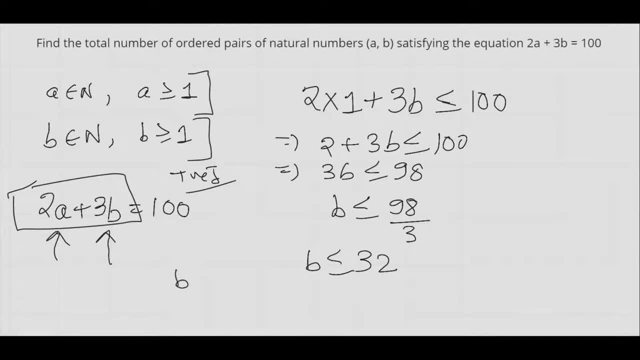 equals to 32.. So B: the range of B is from 1 to 32.. Okay, Now we know the range of B. right Now we can see that since this equation has two here, this will always be even hundred. 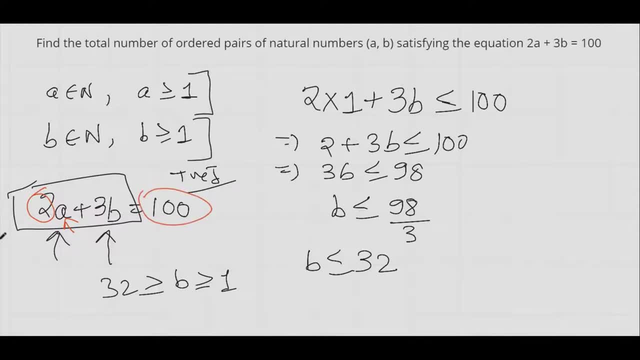 year is also even. So whenever we add or subtract two even numbers, we always get an even number. So this also has to be a even number. Since three is odd, multiplying it with any odd number would give me an another odd number. 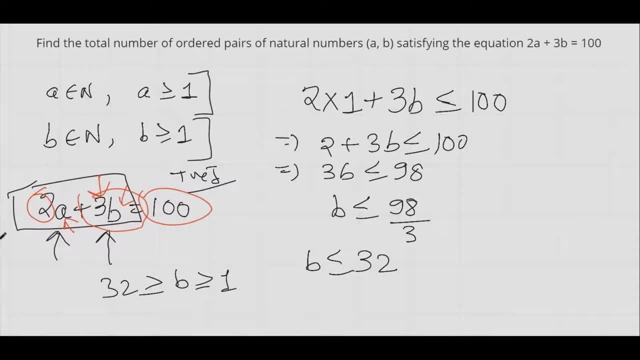 So B has to be an even number, right. So what are the possible values that we can take? 2468, dot, dot till 32.. The count of this numbers is 16.. Now we have the maximum value which we can take. and minimum value which we can take Now, since B is even three, B will also. 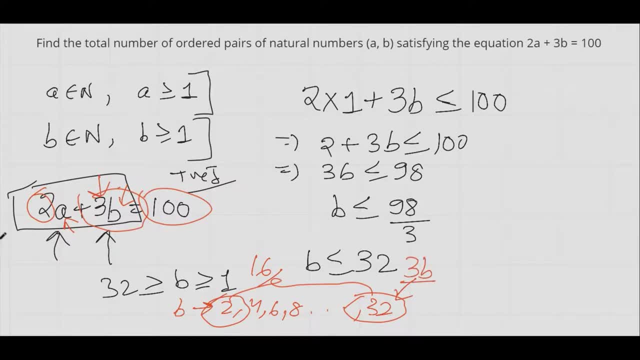 be even Subtraction of two even numbers: 100 and 3B will always be another even number. So 2A will equal to an even number And since it will be divisible by 2, A will always be an integer right Now, since the maximum value of B is 32.. So the minimum value which 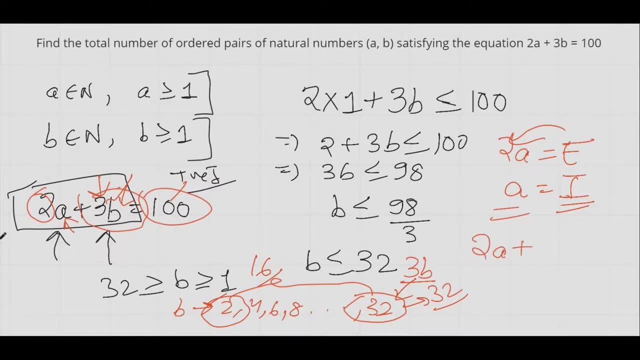 get is: 2a plus 3 into 32 is to 100, right. so on solving this, we will get a as 100 minus 96 by 2, which is equals to 2. so, on taking any other value less than 32, 3b would be less. 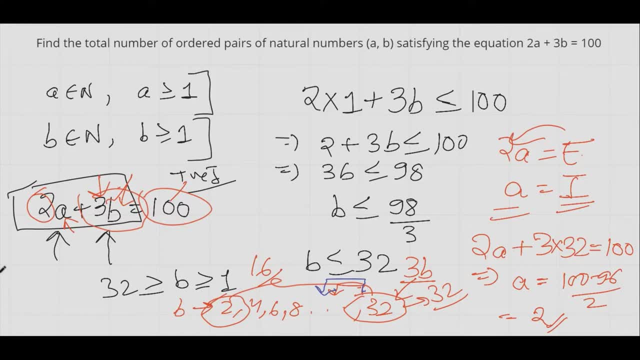 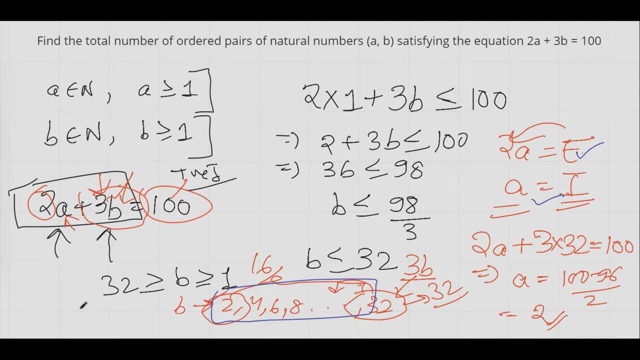 than 96, but it would be an even number. since this, all are even numbers, right? So 2a would be an even number and a would be an integer which would be greater than 2, right? So as b decreases, a will increase, right. Since every value of b is unique, the ordered pair will also be unique as the value of a. 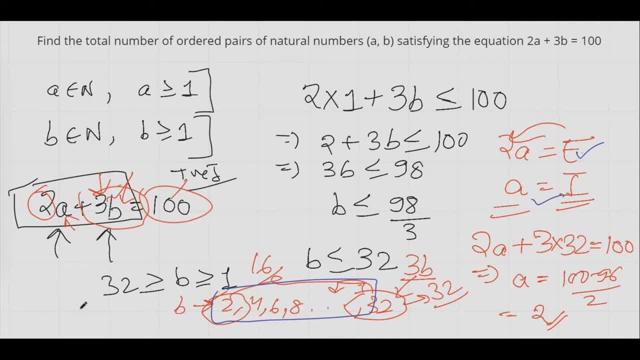 will also be unique, will keep on increasing as b decreases. so total, there would be 16 solutions, right one for each of the value which we can take from this: 2, 4, 6, 8 and 32, so the total number of ordered pairs. 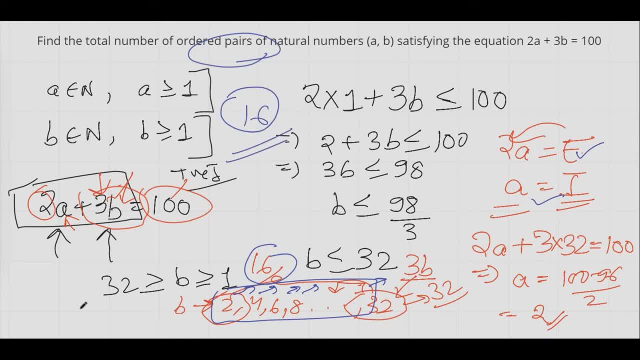 would be 16. if you have any question, please feel free to drop a comment. thank you. 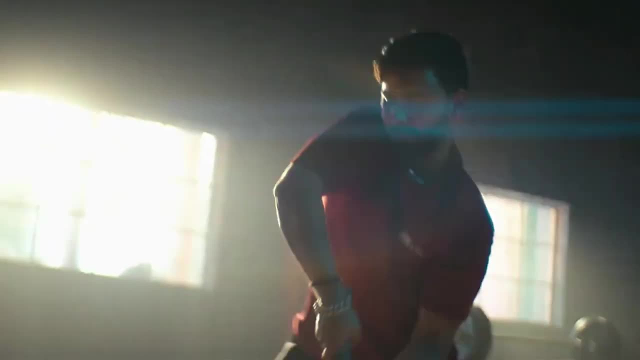 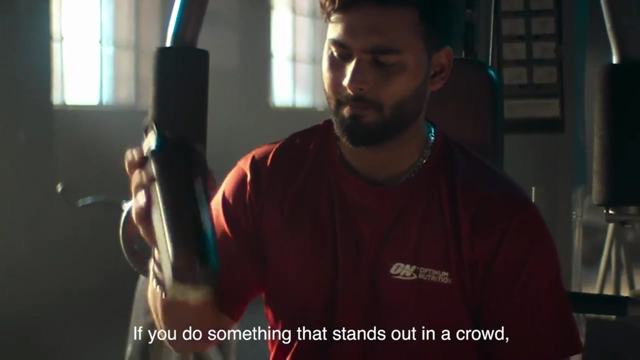 Protein powders have long appealed to people who want to build muscle and become stronger, but they can also help people who want to shed weight. As a convenient and tasty way to increase your protein intake, these powders can be an effective way to support your weight. 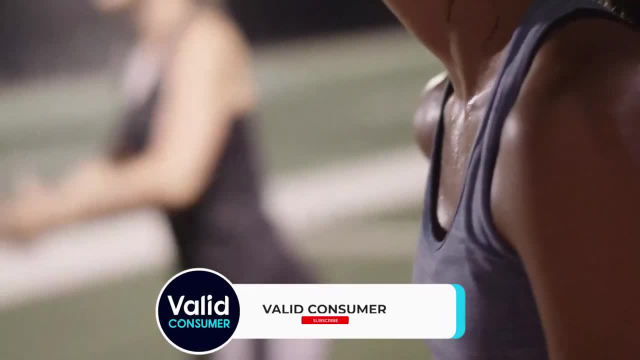 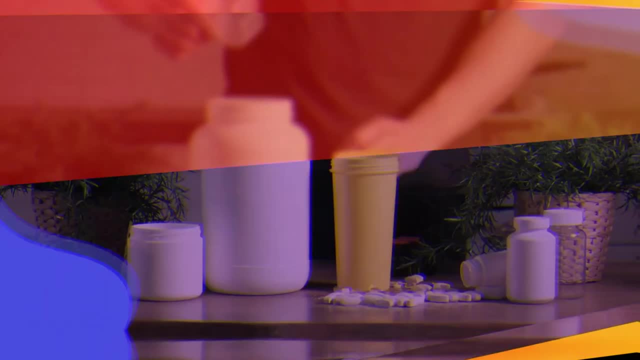 loss efforts. However, with the dozens of protein powder options available, it can be challenging trying to decide which is the best choice for your weight loss goals. We did the legwork and we have listed the top five protein powders and their key features.